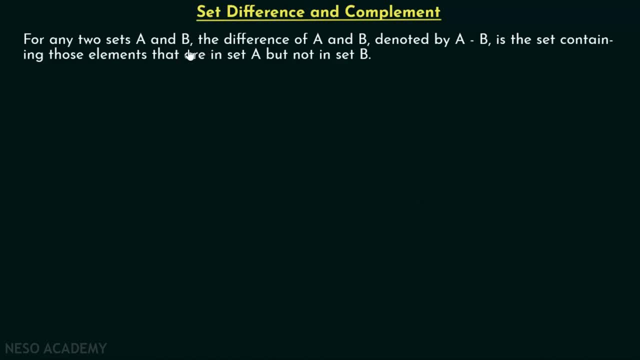 Very simple to understand. We have two sets, A and B. We are talking about the difference of A and B, which is A minus B, and A minus B is the set containing those elements that are in set A, only in set A, but not in set B. 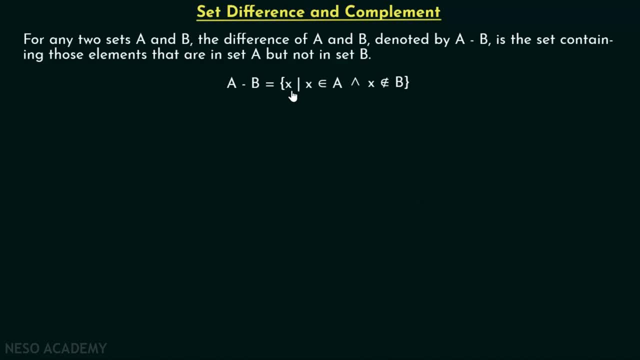 In other words, we can say that A minus B is a set of all X, such that X belongs to A and X does not belong to B. Okay, now we will see when diagram representation of A minus B, and this is how it looks like. 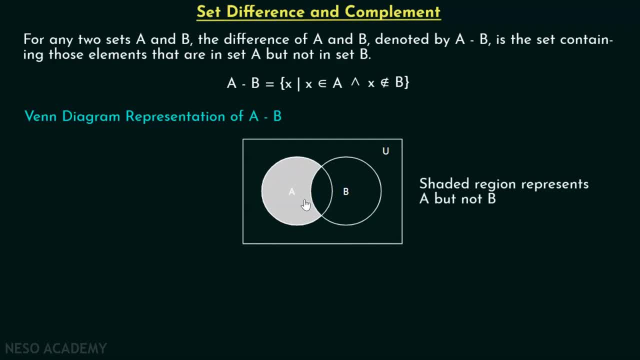 Here, this shaded region represents A but not B. okay, We can't include this portion, this area? okay, Because if we include this area, then this means we are including some elements of B as well, which is incorrect. right, Because we are talking about only A and not B. 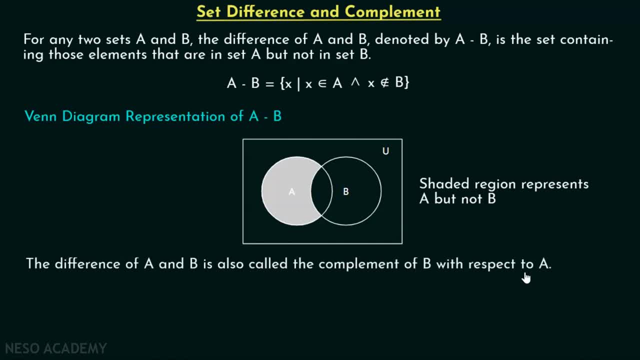 So the difference of A and B is also called the complement of B with respect to A. okay, Now here is one example. Let's say A represents this set and B represents this set. There are three elements in set A and there are three elements in set B. 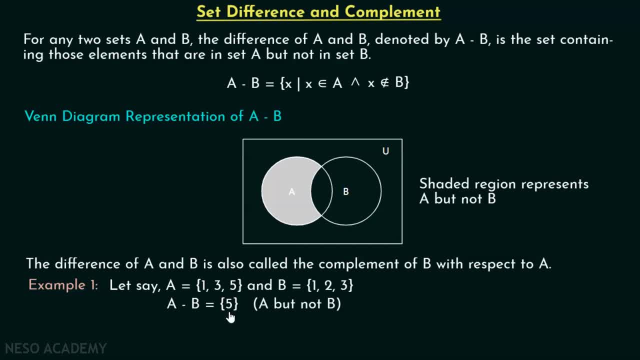 A minus B is nothing but a set containing only one element, that is five. Because here you can see, in set A we have one, three, five, and in set B we have one, two, three. One, three is common between A and B. 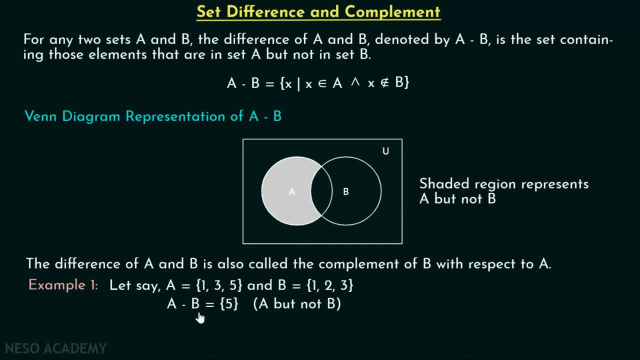 We can't include this in A minus B. That is why only one element is there in A minus B, which is five. right, This is A, but not B. okay, Now let's consider one more example. Let's say: A is not B. 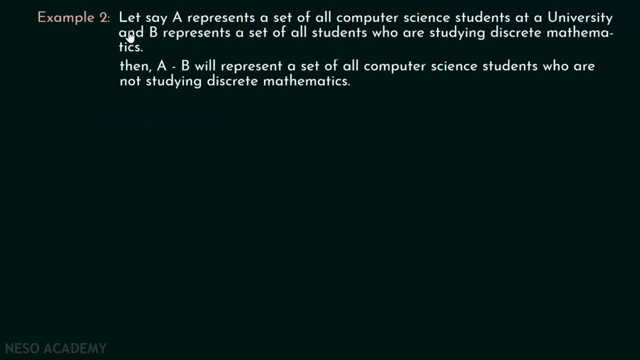 Let's say A represents a set of all computer science students at a university and B represents a set of all students who are studying discrete mathematics, Then obviously A minus B will represent a set of all computer science students who are not studying discrete mathematics. Please see this. 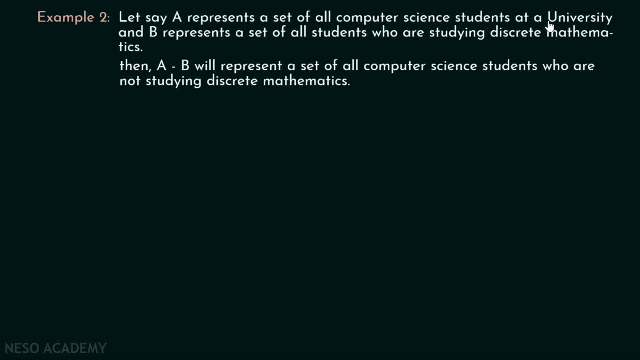 A represents a set of all computer science students at a university and B represents a set of all students who are studying discrete mathematics. So it is clear that A minus B must include all students who are studying computer science But they are not studying discrete mathematics. okay. 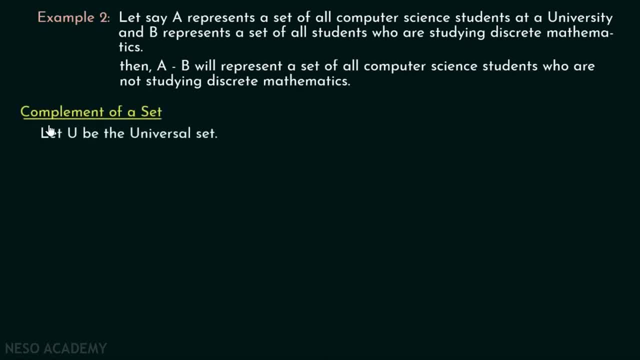 So this is important for us to understand. Now, what is complement of a set? Let U be the universal set, okay, We can also represent a universal set by capital E, but here I am representing universal set by capital U. This particular notation you can see in many books, okay, 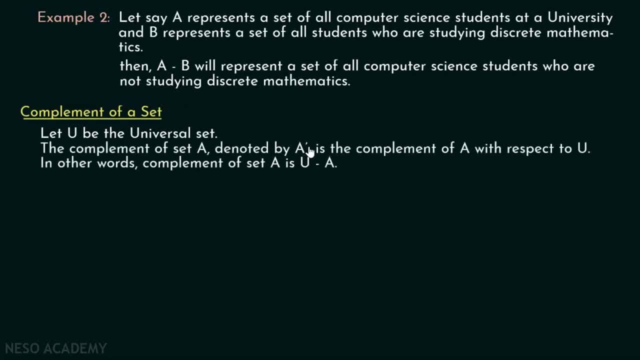 The complement of set A, denoted by A complement- this dash over here- is the complement of A with respect to U. In other words, complement of set A is the complement of A with respect to U. The complement of set A is U minus A. 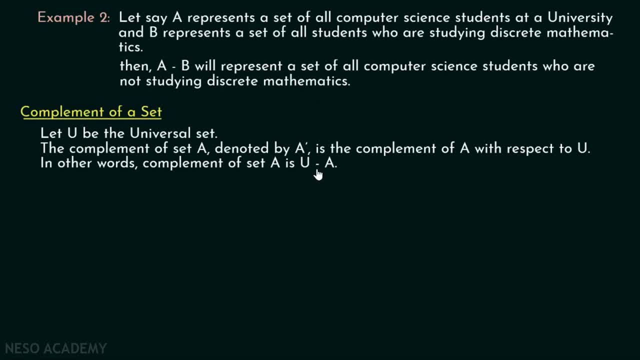 Very simple. So subtract A from U, which means there must not be any A. okay, That means everything under consideration except A. So A complement is nothing but a set of all X, such that X does not belong to A. Isn't that simple? 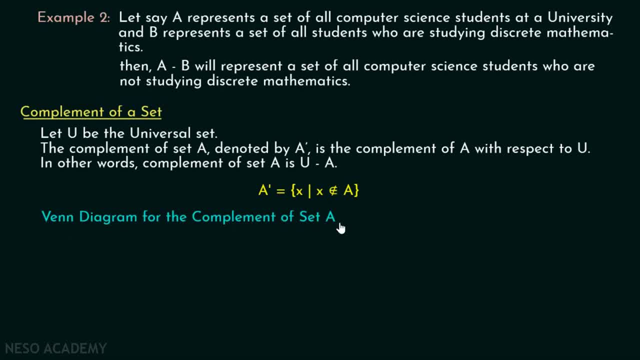 Now let's see Venn diagram representation for the complement of set A, And this is how it looks like. right Here, this rectangle represents universal set and this circle represents set A. Here, shaded region represents A complement, Isn't that so? 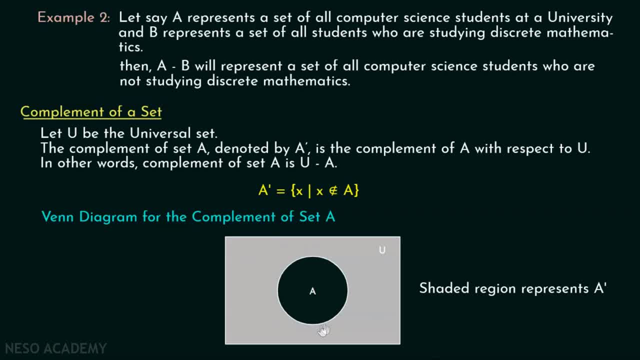 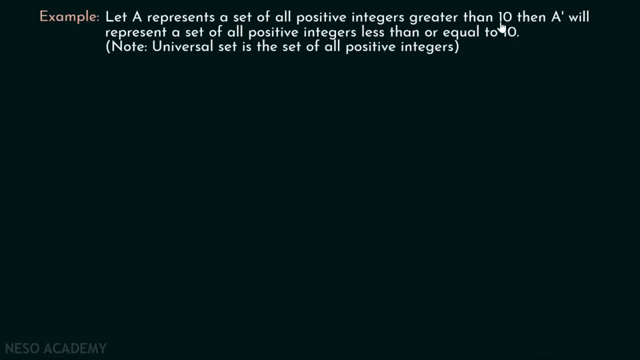 Here everything is included except A. This is A complement. fine, Here is one example: That A represents a set of all positive integers greater than 10.. Okay, So A represents a set of all positive integers greater than ten. Then A complement will represent a set of all positive integers less than or equal to 10.. 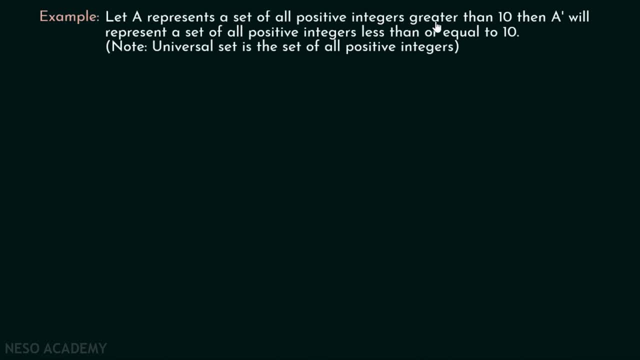 Isn't that so? Because A represents a set of all positive integers greater than 10.. Right, Obviously, A complement will include all positive integers less than or equal to 10.. And please note that universal set is the set of all positive integers. 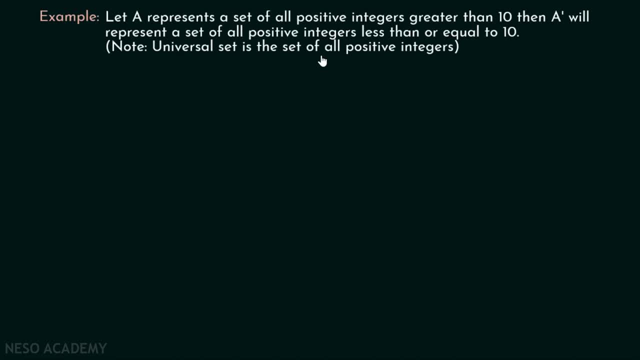 Right, Here I am considering the universe of discourse as set of all positive integers. Please note this down, Okay. That is why A complement will represent a set of all positive integers less than or equal to 10.. Right, And this is how it looks like. 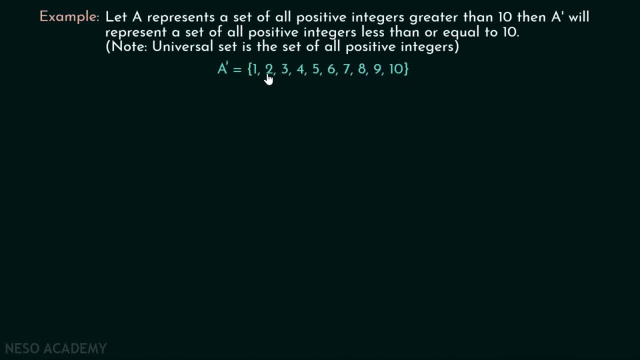 A complement is nothing but a set of all positive integers less than or equal to 10.. 1,, 2,, 3,, 4,, 5,, 6,, 7,, 8,, 9, 10.. All these elements are included within this set, Okay. 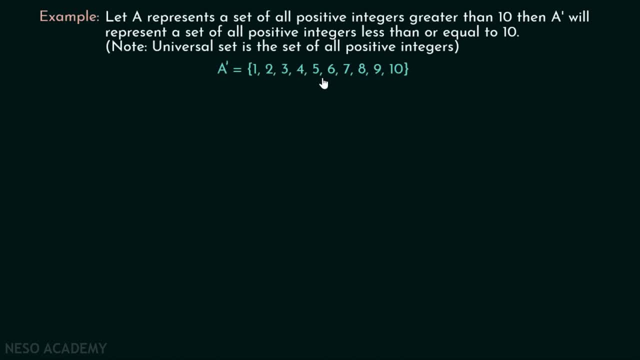 Okay, friends, this is it for now. Thank you for watching this presentation.